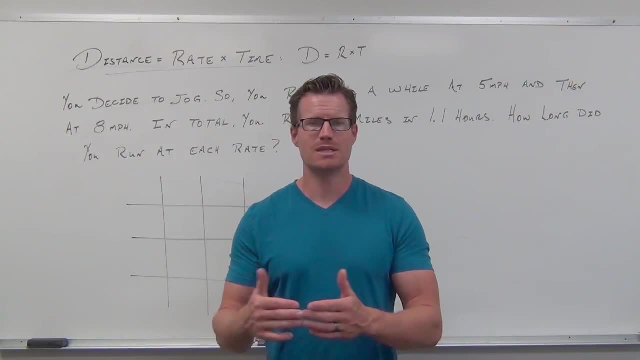 going to go Well. 60 miles per hour means in every hour you have gone 60 miles, So 60, and then another 60, and another 60 or three times 60, that's 180 miles. That's what distance equals rate times. 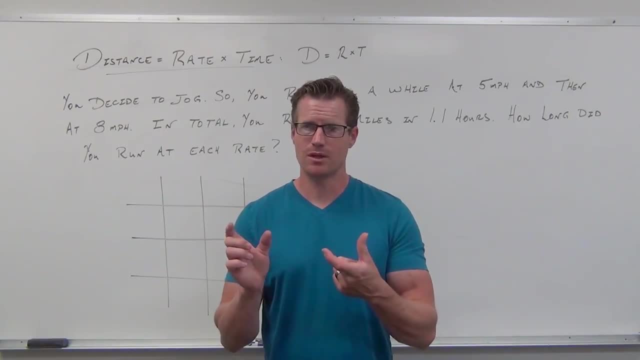 time does. for you, The distance is going to equal the rate that you're traveling. for the time that you're traveling, It kind of takes for granted that you're going to study speed. So if we're not going to study speed, that's outside of the realm of this. distance equals rate times time problem. 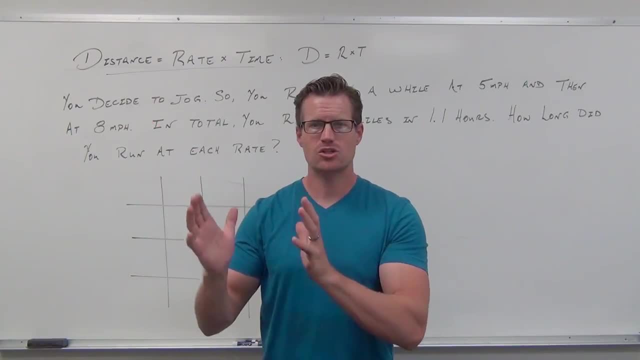 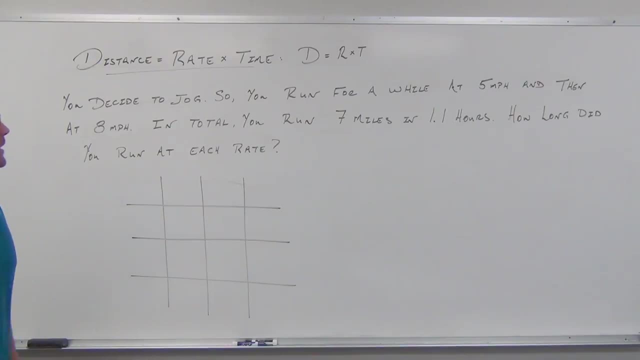 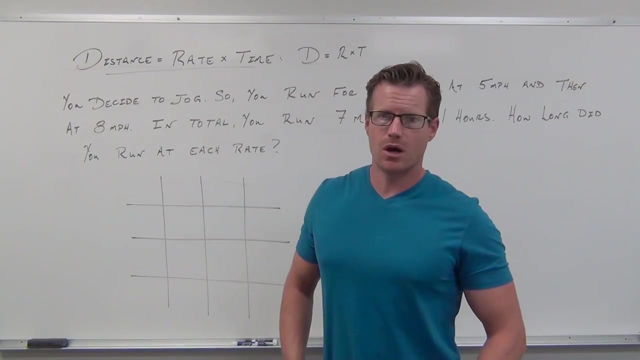 So we have a distance equaling how fast you're going for how long you're going. We can use that. So let's say that we have our example here and you decide to go for a run. So you're jogging long and you jog five miles an hour for a little while, and then you step it up and you jog eight miles an. 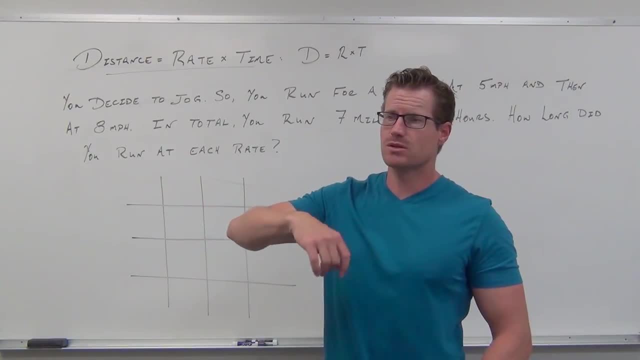 hour to wherever you started from, and you've gone seven miles. It took you 1.1 hours. So we know a lot already. We know how long we ran. We know how long we ran it for. What we don't know is how long we. 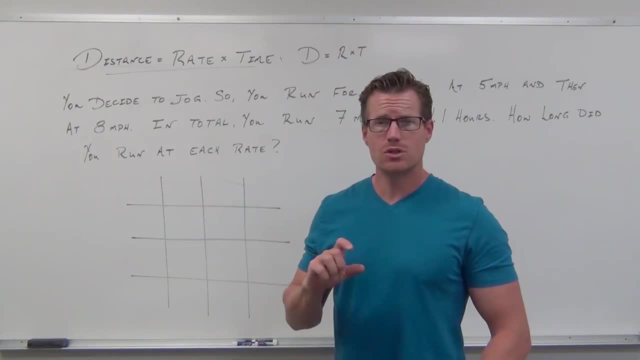 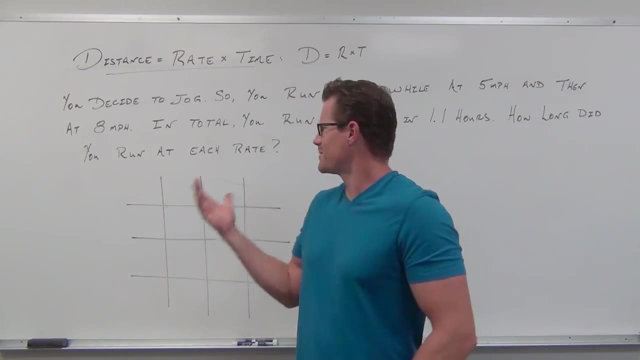 ran each jog for each segment. So I'm going to give you a tool, a graphic organizer, to help you with this, because at first glance we read through these problems. I don't know. We're supposed to guess and check. I guess, Well, that's really slow. It works sometimes, but it's really slow. 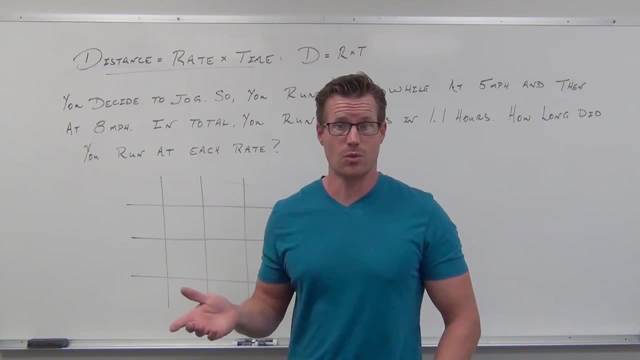 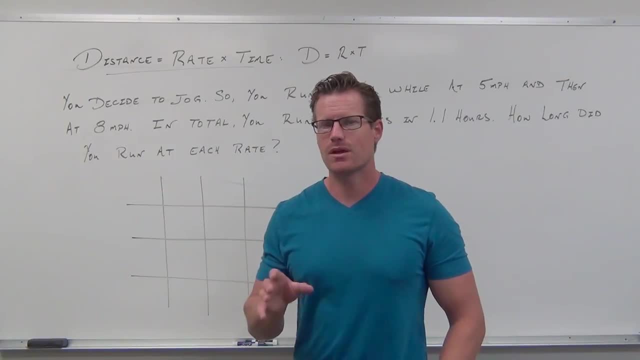 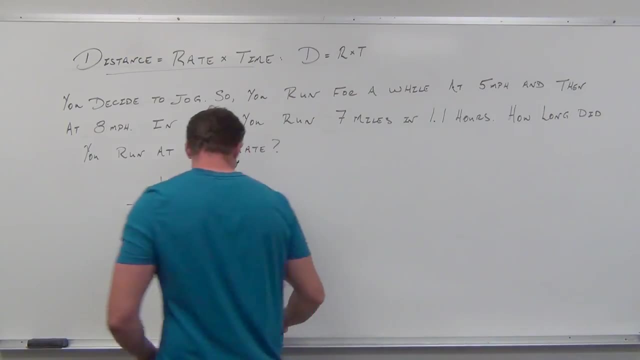 how to do the math. So let's write down everything that we know in a table that organizes our information for us. So most of the time, what we're going to do is we're going to start off and we put the scenarios on the left-hand side- What's going on here, And then something that 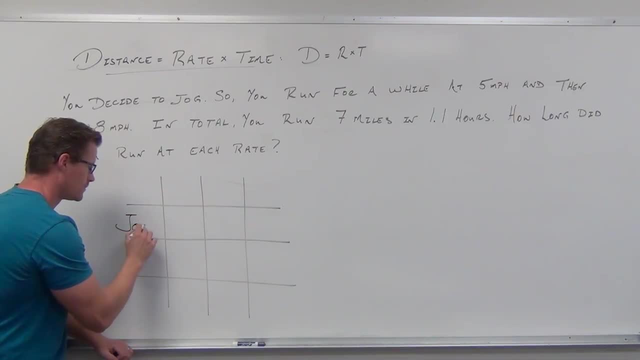 relates them up here. We had two jogs. We had, let's say, jog one, Jog two, And then we had a total Up at the top. we know that we had- and this would be part of the formula aspect of word problems. So we've read it. We'll probably read it again very carefully in a 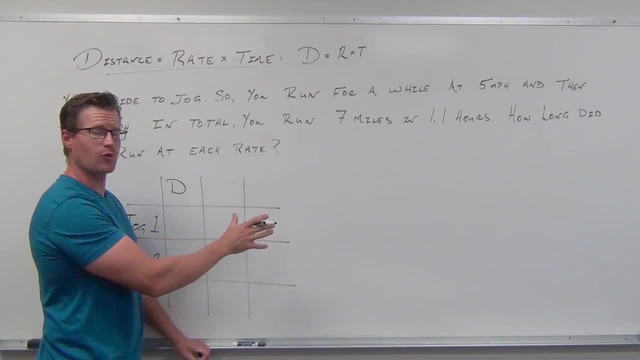 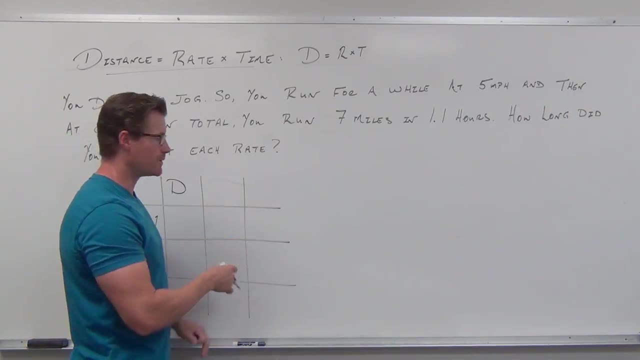 minute. We have a sort of a picture of graphic organizer and a formula going on. This is going to create the verbal model for us. After that we'll fill in the variables, We'll get our equation, We'll solve it. But this is the hardest part. 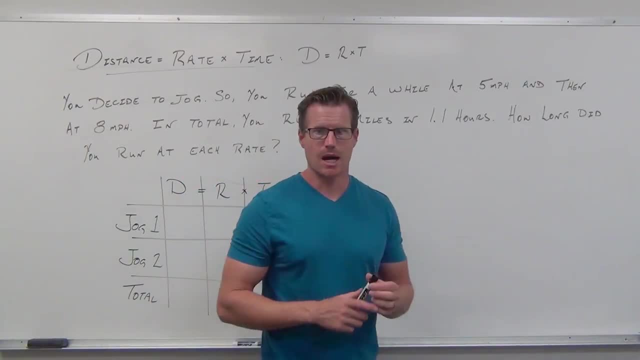 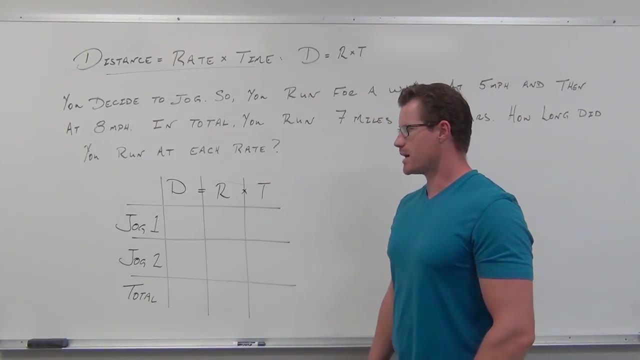 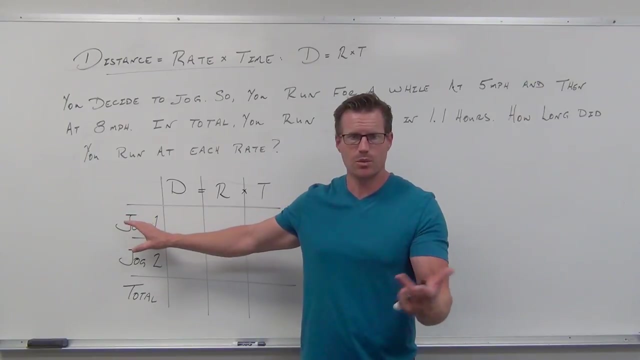 Any time you're moving through space and time, you have distance equals rate times time if your rate's continuous. So we have that here. So our distance equals rate times time. Put your scenarios here: How many different rates you ran, how many different jogs you did, whatever it was. 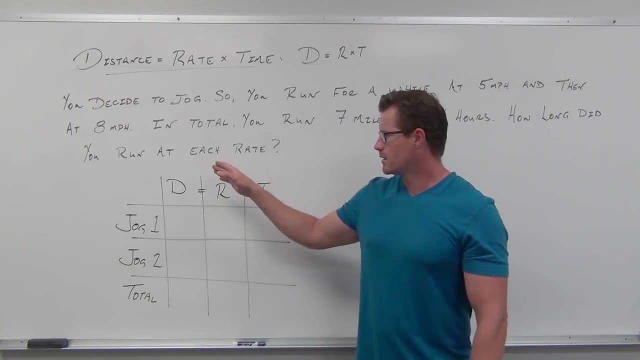 Jog one, jog two and how much you totally did. Distance equals rate times time. There's three things that are related to any distance problem: The rate, the time and the total distance. Write down everything, Everything you know. So we're going to read the problem carefully right now. We're going to write down everything that we know. 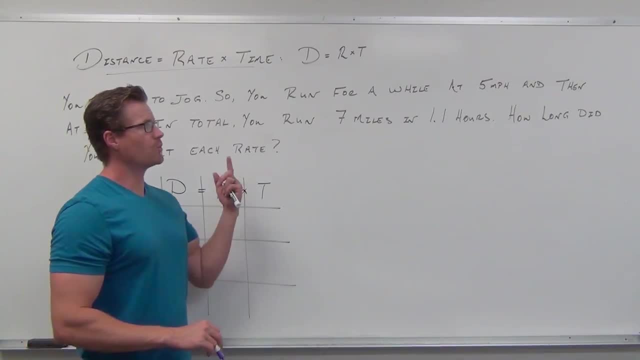 So we're running. OK, we've got it. First jog: we jog at five miles an hour. That's a rate. So right here in our little matrix we have jog one, five miles an hour, And then we run at eight miles an hour. 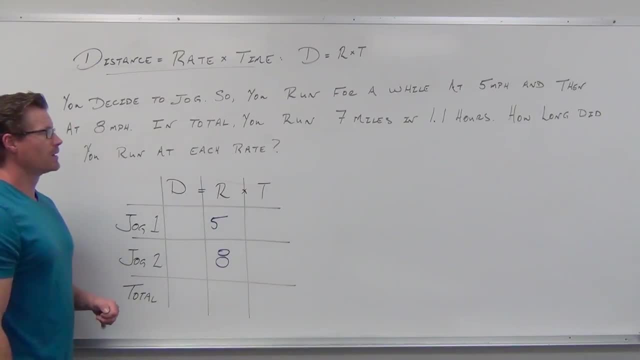 Let's call that jog. two In total. all right, we got a total. We ran seven miles And we ran for a total of one point one hours. How long do? OK? so that's the question. So now we're going to go through and make sure we don't miss anything. We have two. 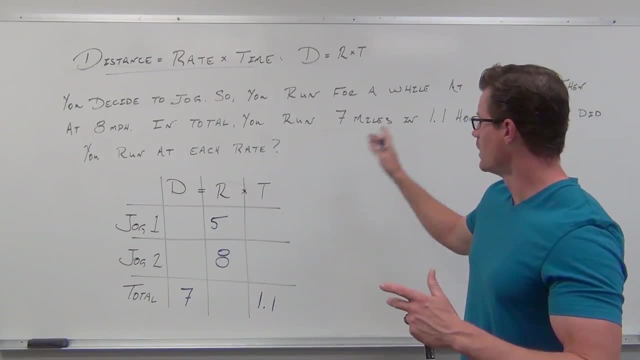 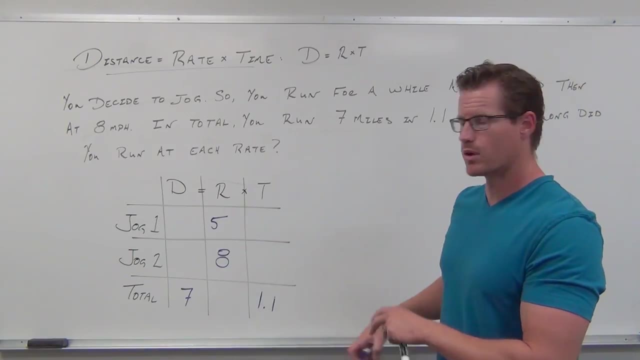 jogs. we got two jogs. We had a distance, a rate and a time. OK, let's fill that out. Jog one was five miles an hour. Jog two was eight miles an hour. We had a total of seven miles and we had a total of one point one hours. It also helps if you put that this is: 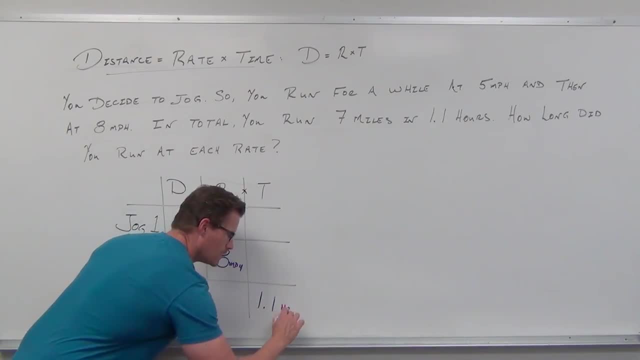 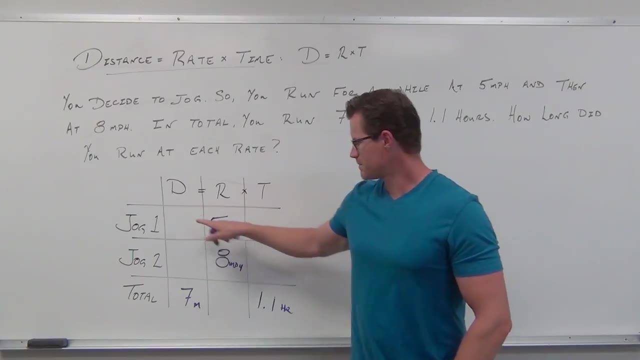 your rate, your total miles and your hours, just so you know what you're dealing with. Now the rough part is figuring out what goes here and here. You see if we can figure out what goes here. this is the big part. 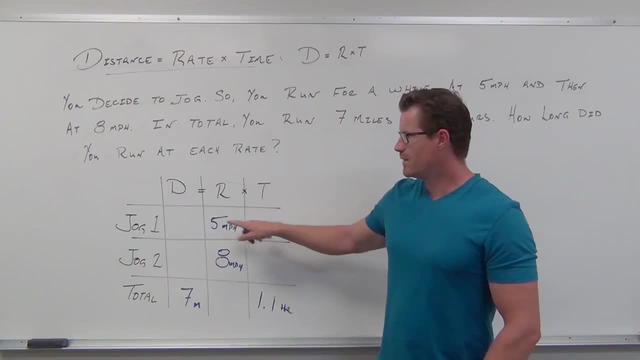 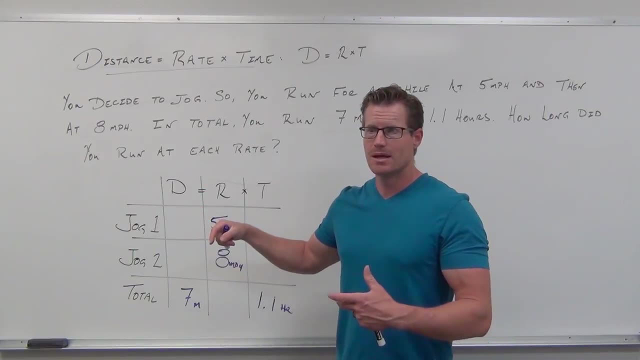 here. if we can figure out what goes here and here, then these columns really work together. And I'll talk about a little bit after we're done with this example, how you can change this around to illustrate more examples. okay, But if you find a rate and a time, you automatically know. 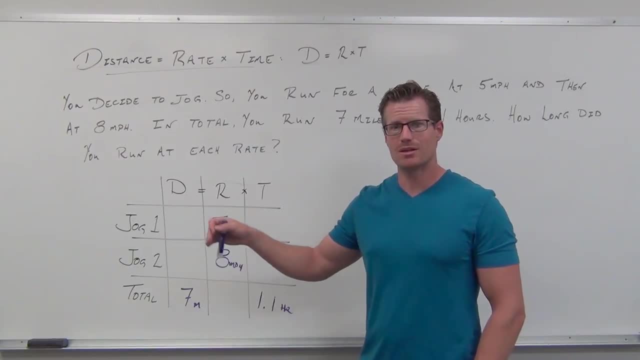 a distance. If you find a distance and a rate, you automatically know a time. If you find a distance and a time, you automatically know a rate. So, given any two variables, you know the third one in this. So, for instance, let's say that this was, it's not going to be five hours, six hours. 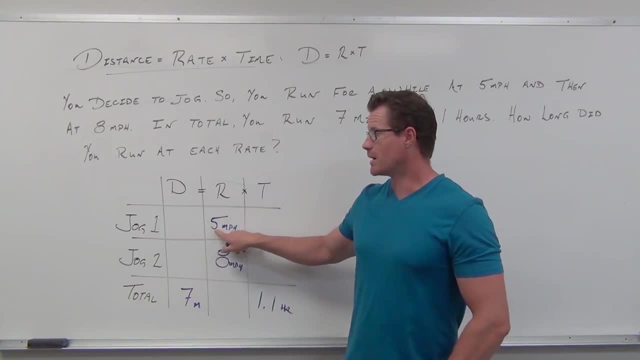 but I'm going to make it up right now. Let's say that they ran five, or you ran five miles an hour for something. Six hours, That's 30 miles. If you know this, you can just multiply. that's the key here. 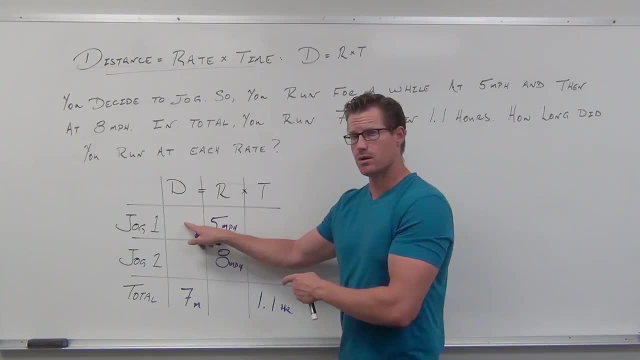 multiply these two columns to get that one. So to get that box. Distance does equal rate times time. That's great, but we still don't know this. So let's think carefully. Do you know how long this person ran for job one? Do you know how long the person ran for job two? 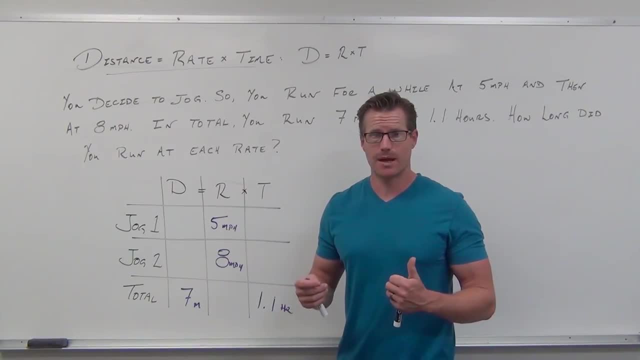 You're going to have to pick one of the two. If you wanted these to be a variable, it doesn't matter. What does matter is that you understand we are in linear equations and, as we discussed in the approach to problem solving, you can only use 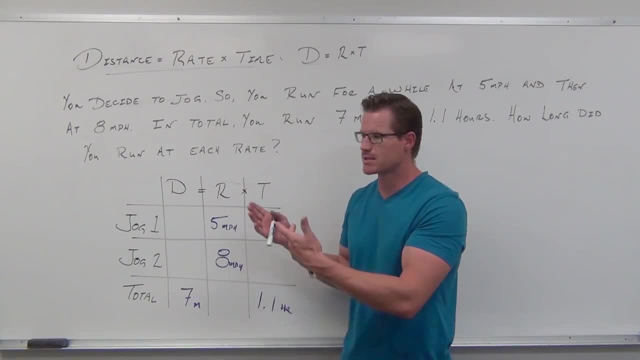 one variable, So call whatever one. you want a variable, It doesn't matter, but in the other box you have to relate it. Now, here's the key. okay, Don't miss this. Get this. Do you understand that? 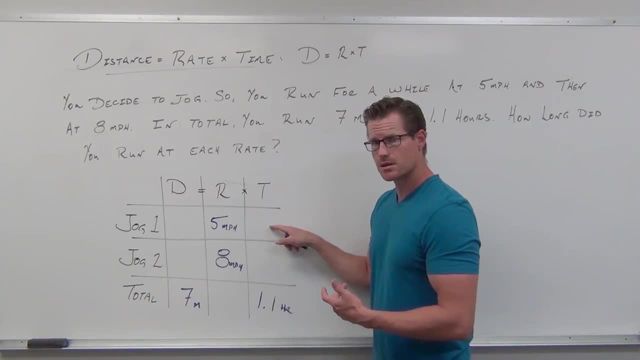 the amount of the time the person ran here plus the amount of the time the person ran here has to equal 1.1 hours. Do you get that? Yes, So you're going to have to pick one of the two, So let's. 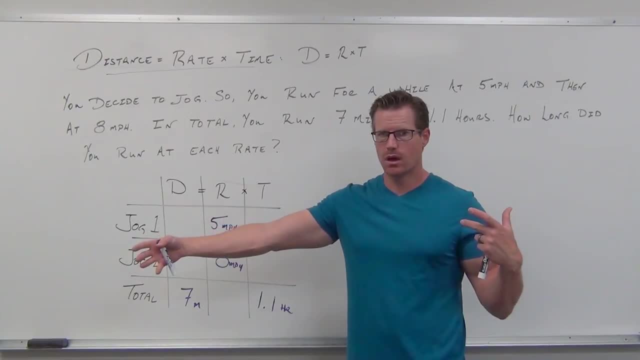 think carefully: If you ran a total of 1.1 hours and you ran a portion of it- this speed and a portion of this speed- well the times that you ran they got to add up. You can't run for two hours plus. 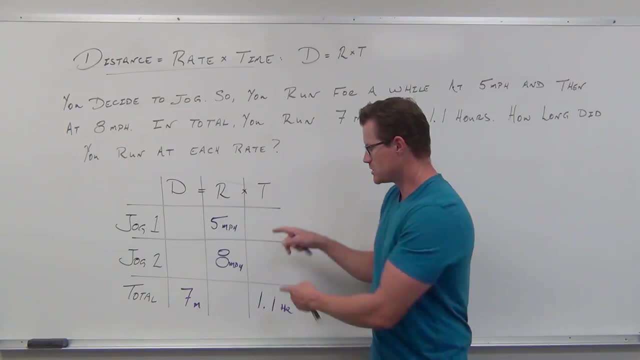 five hours and get 1.1 hours. It doesn't make sense. These two have to add up to 1.1.. The time you ran here plus the time you ran here has to equal the time you ran there, If you guys get. 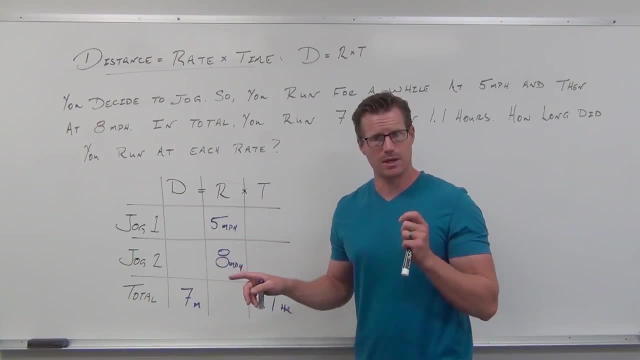 that this is not hard. Think through this before you go any further. Make sure you understand that these times have to add a total time. Time you ran for one, time you ran for two has to add up the time you ran in total, Because if you get that, check this out, It's pretty cool. Call either one. 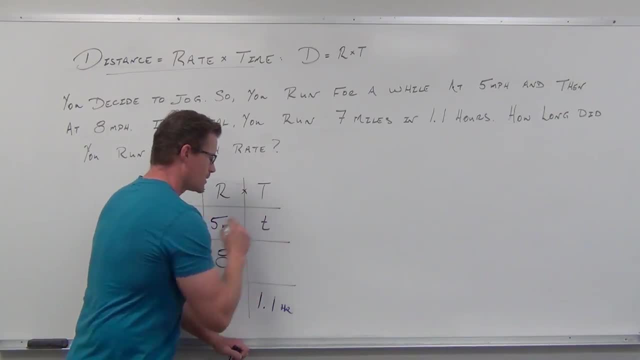 of these a variable. You know what I'm going to use. I'm going to use t to stand for time. I don't know what that time is. It doesn't matter which one you choose. What does matter is this: If you 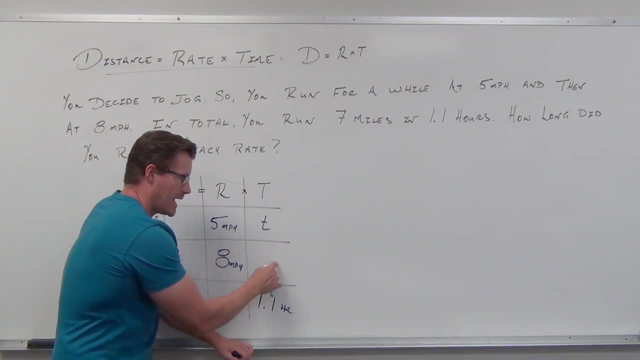 because we're going to find this out right now. If you really get that, these two have to add up, call this a blank space, like Taylor Swift does. Call it whatever you want, I don't care, We're going to call it what you call it, But understand this. This is pretty neat. Understand that t plus blank. 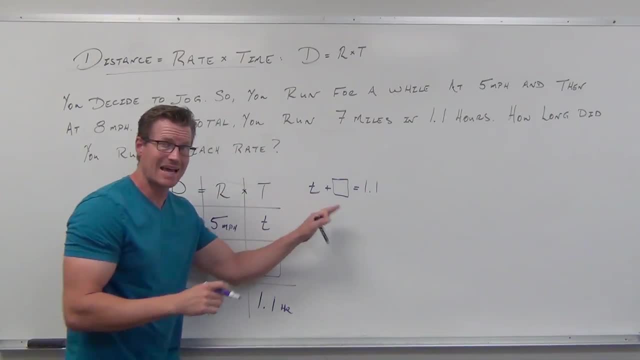 space, if you want, equals 1.1.. If you get that, that's awesome. You understand the idea. Your times have to add up. t plus I don't know has to add up to 1.1.. Solve for that, If you solve. 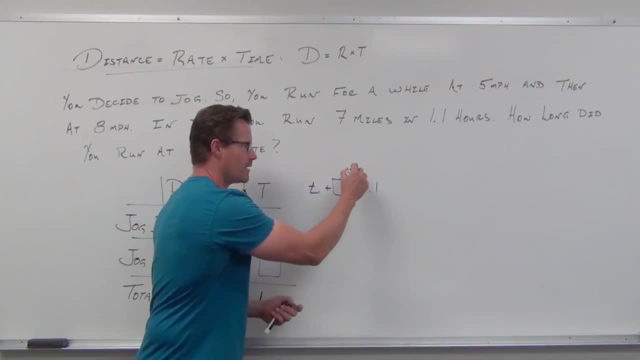 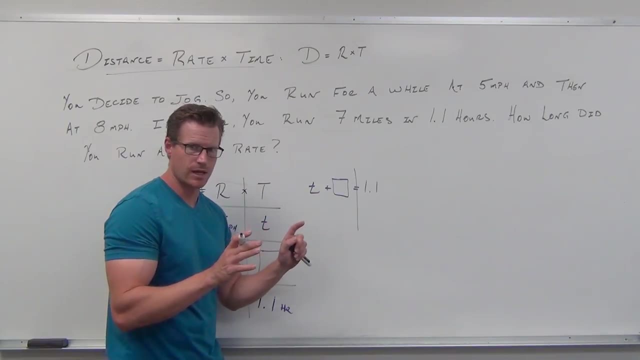 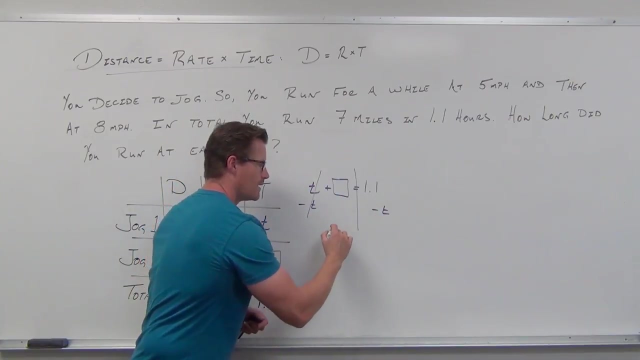 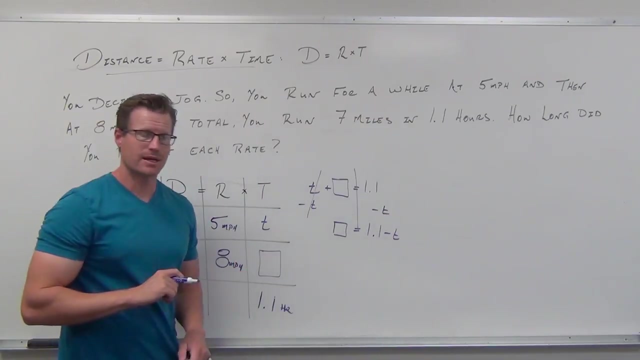 for that? what do you mean? solve for it? Hey, that's an equation. Get this by itself, Remove it completely, Not divide Subtract. It's connected by addition Subtract. If you subtract that t, then we automatically not like terms, we automatically find out what should be in our 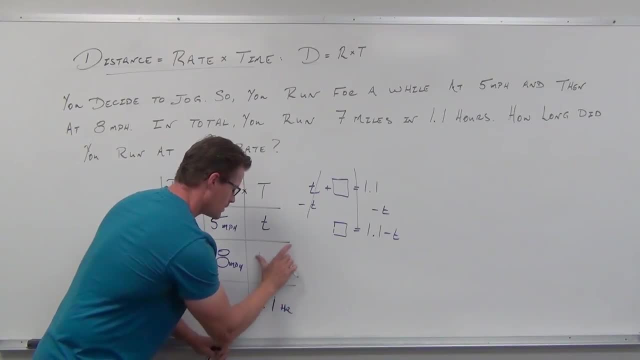 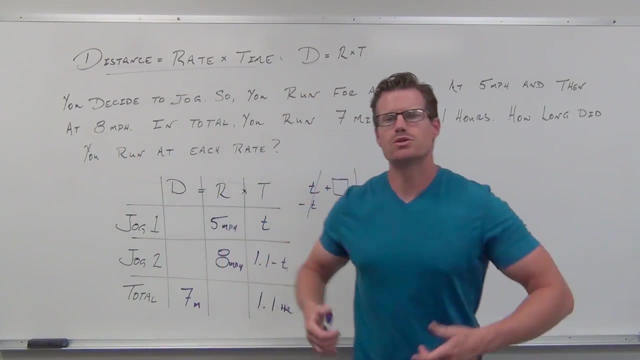 blank space. what should be in that box? Now, let's think logically through it. If I told you that you ran for 1.1 hours, you would have done the same thing. You would have done the same thing and I said: hey, that's 0.1 hours. 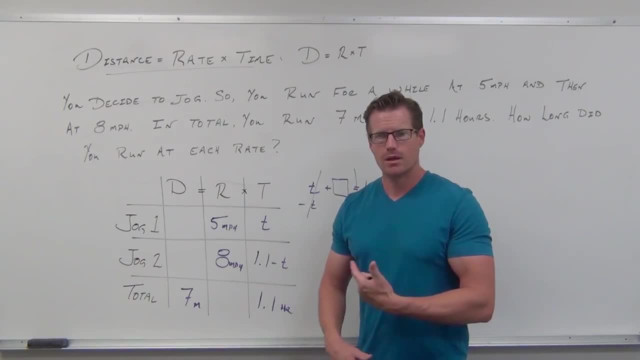 To find the missing spot you'd have to subtract it from 1.1.. That's the idea here. It's saying if you ran for a total, you're going to have some. You'd have to take this something away from the total to figure out what's left. 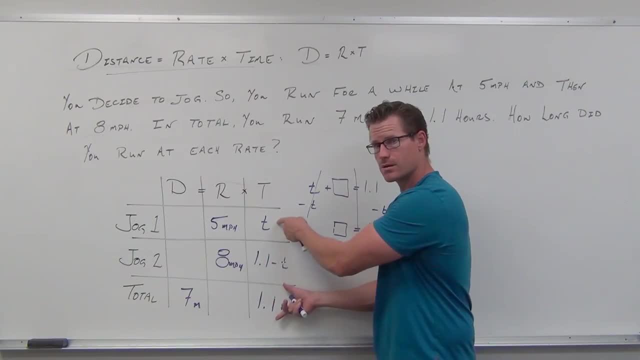 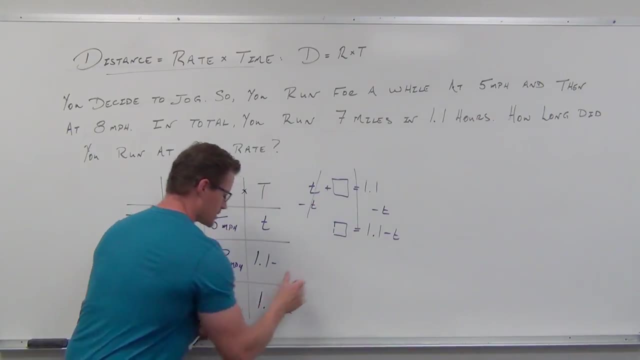 That's the idea. You have a total. You're taking up some of it here. Take it away from the total to figure out what's missing. That's what the math does for you. What's even more equally interesting is that if you add these up, it does equal 1.1.. 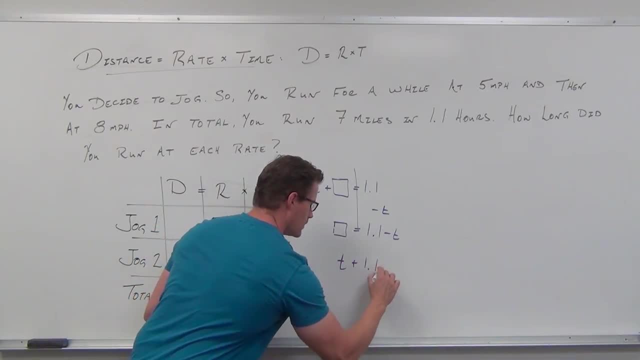 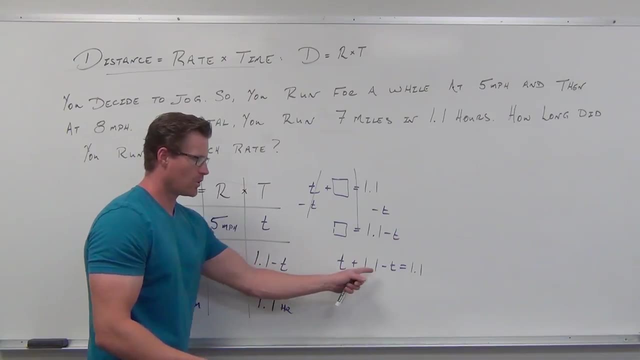 Try it if you want to. It's almost a trivial statement because it has to work. It's how you created it: t plus 1.1 minus t, t minus t is gone. 1.1 equals 1.1.. 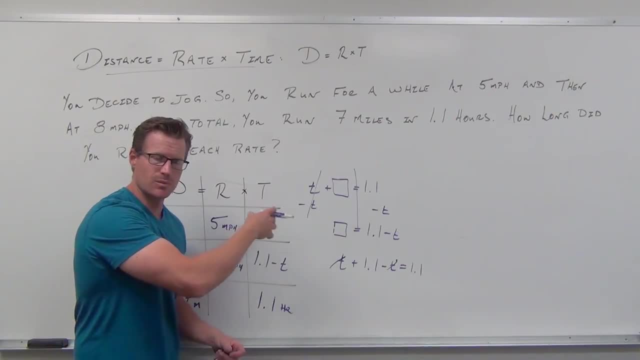 It does work. That's pretty cool. This is a hard concept for a lot of people. If you're not quite getting it, look through it again, Listen to it, Do it at least one more time and then try it for yourself. 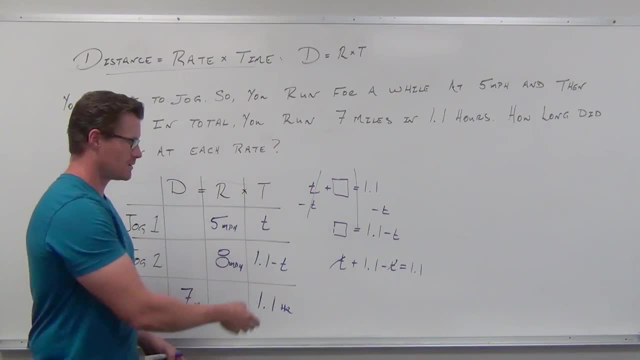 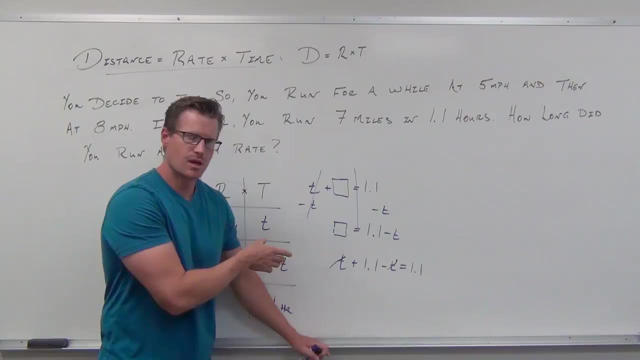 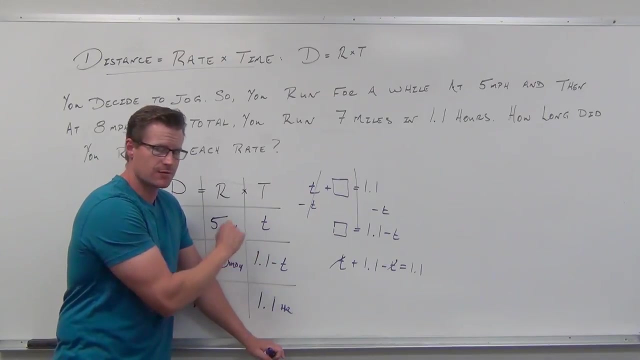 See if you can do this whole blank space idea to get the missing box. This is what makes a lot of these problems possible: is taking a total using a variable you create and relating the missing piece back to that variable, because we can only use one variable. 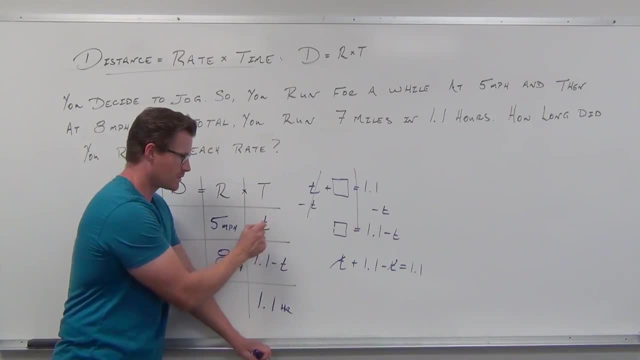 We start with a total, We go okay. well, this is something I don't know, This is something I don't know, but I know that these two have to add up. If these two have to add here, then this one minus this one has to be that one. 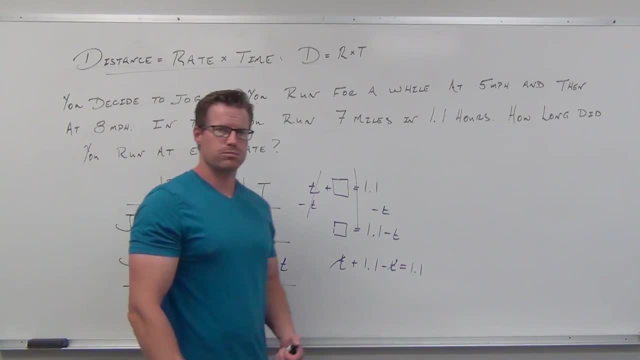 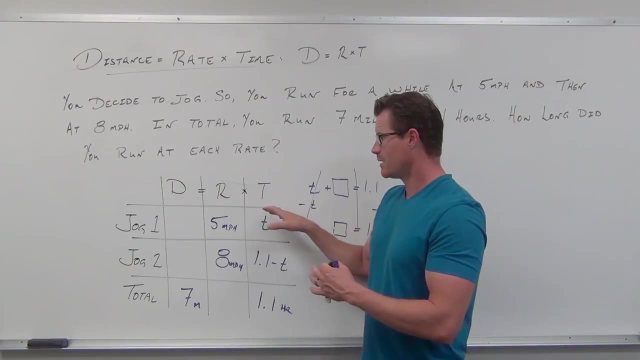 It has to be the missing piece. That's what that math said to us. You're almost done. It doesn't look like it, but you're almost done. You see, we have a rate and we have a time. If rate, times, time equals distance, then we go this way and we can fill out this distance. 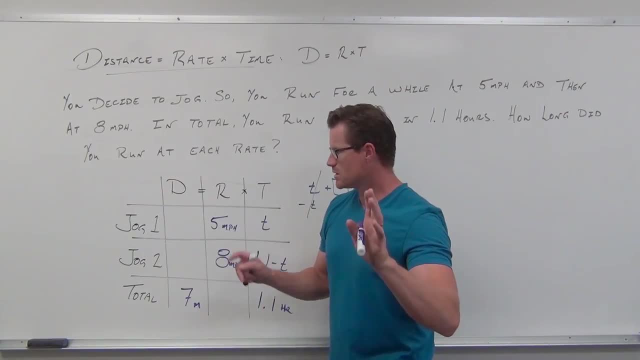 One more thing before we do. I just want you to get this also: Do you understand that Whatever you ran here, how far you ran here plus how far you ran here, is going to equal your total? If you ran three miles here and four miles here, you have to add up to seven miles. 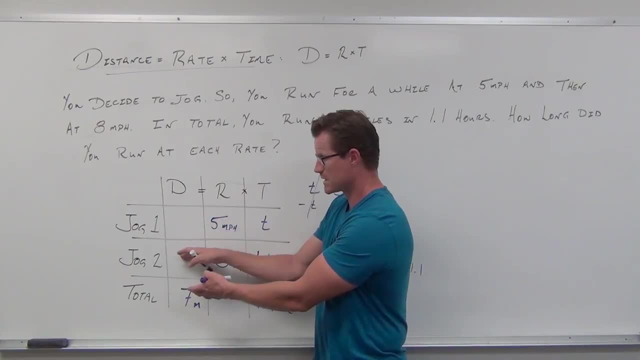 These things have to add up here. If this is two, this has to be five. If this is one, this has to be six. These have to add to seven. The amount that you ran in one plus the amount that you ran in two has to equal the total. 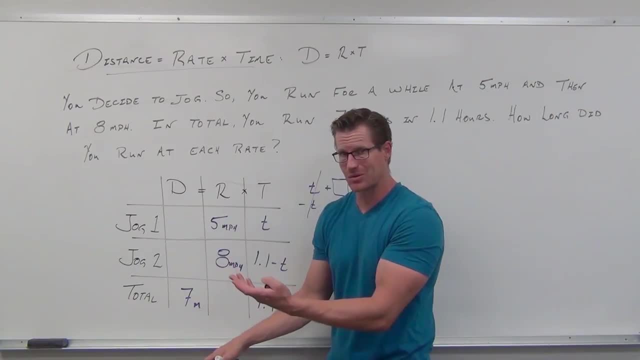 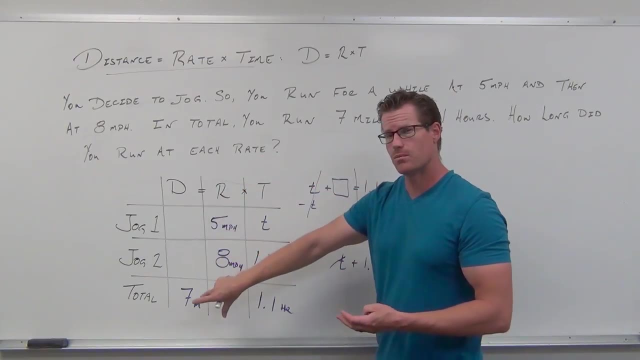 Whatever we get, we can add this up. That's kind of cool. This matrix is starting to hold. It makes sense. We fill out all of our information. This is your little 10-second recap. Fill out what you know, Use what's given to you to create some sort of a relationship with one variable. 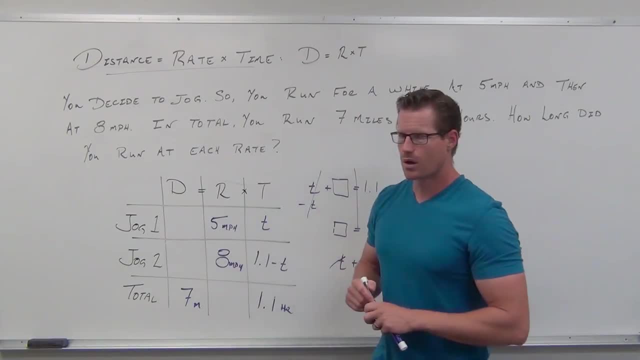 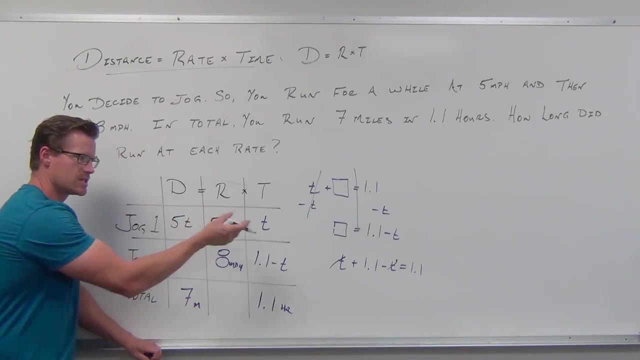 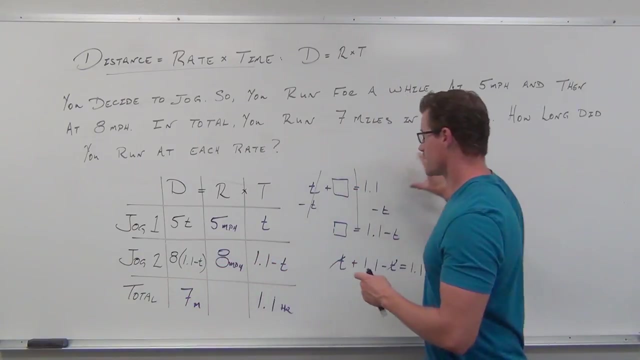 After that, use another column by multiplication or whatever you're given. Five times t is five t, Eight times this whole amount. It's eight times 1.1 minus t. Now we know that our distances have to add up. I'm going to move over here. 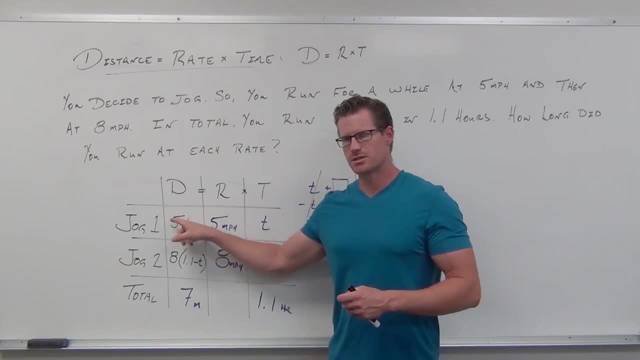 This column basically says it doesn't look like a distance to you. Look at the formula: Rate times. time is a distance. Five miles an hour for five hours is going to be 25 miles. That is a distance. So is that one? 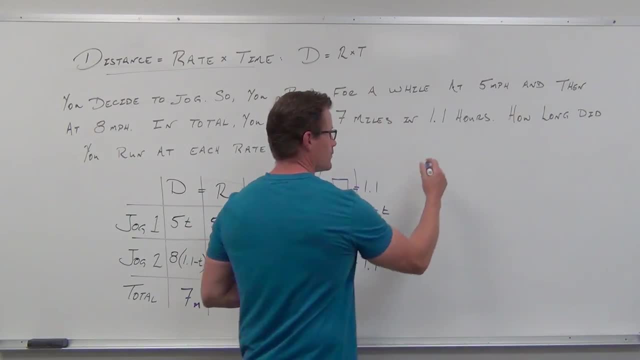 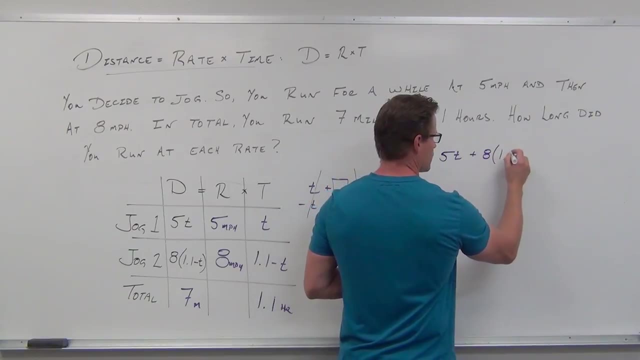 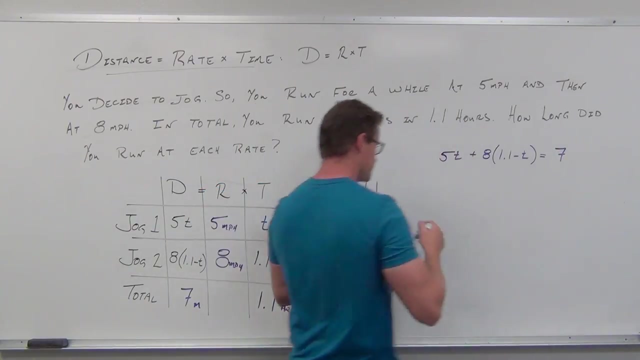 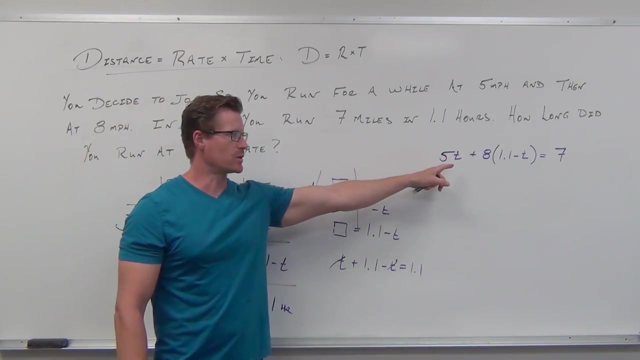 These two distances have to add to your total. We have our first distance, Our second distance And they have to add to the total. What's easier That? It's a linear equation. It's got a decimal in it, but who cares? 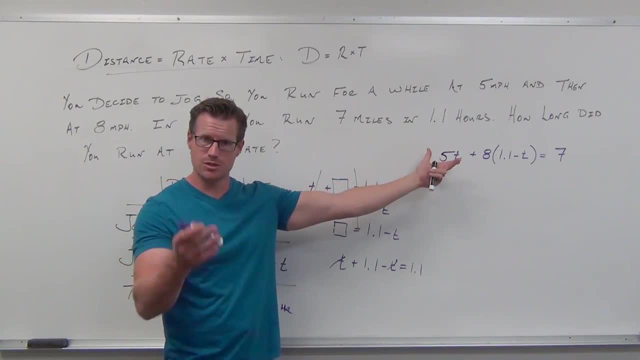 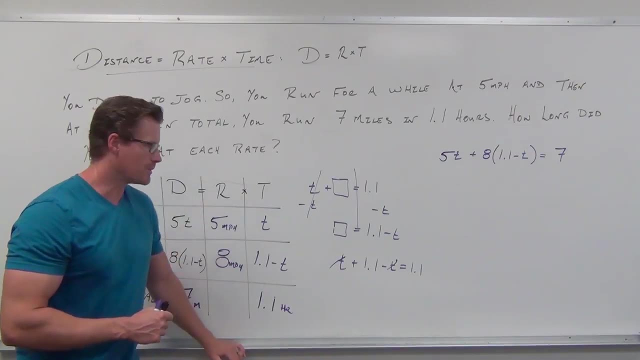 It's got some distribution, It's got some like terms. It's pretty easy to solve because you know what you're doing already. This is the hard part. The hardest part is figuring out how to start honestly, And what it does is it. 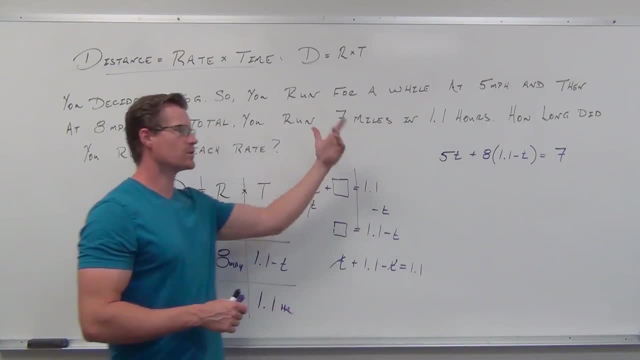 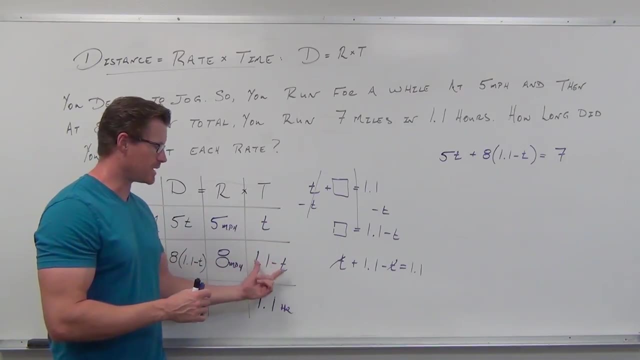 It takes what you're asked for- how long did you run- and that becomes your variable. Relate the missing box- or whatever you want to call this, the missing blank space- to that variable. Then use another column to add up. 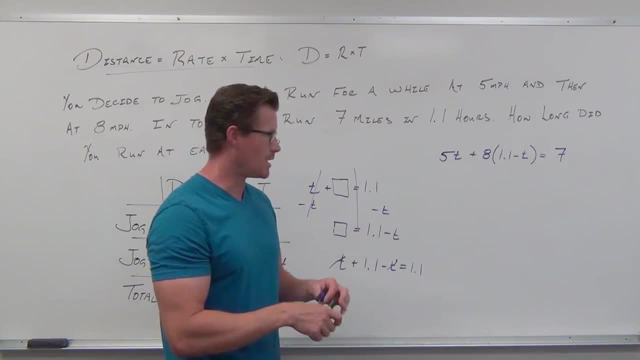 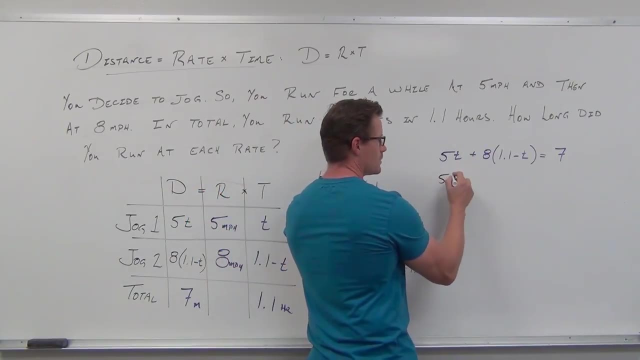 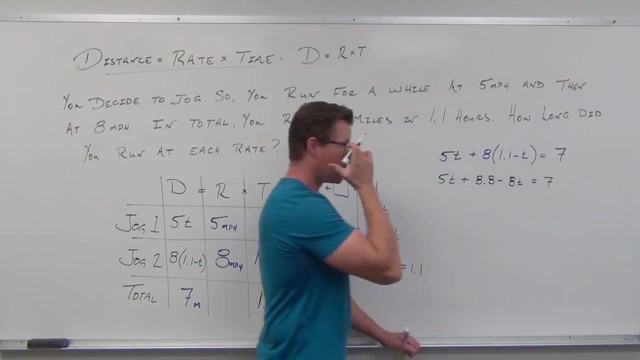 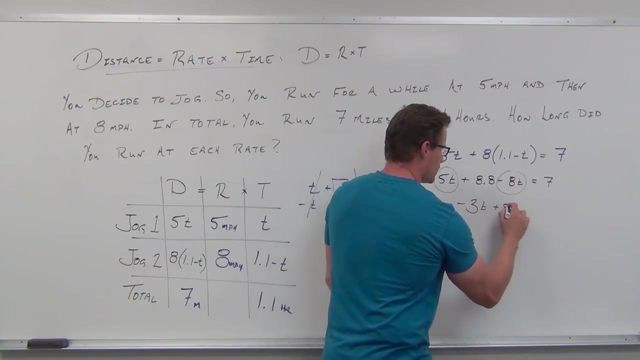 It's usually a multiplication or a division. concept of distance equals rate times time. So now let's solve it. Maybe stop this and solve it on your own, So we would distribute. We check for some like terms and we have some. Our variable is right there. 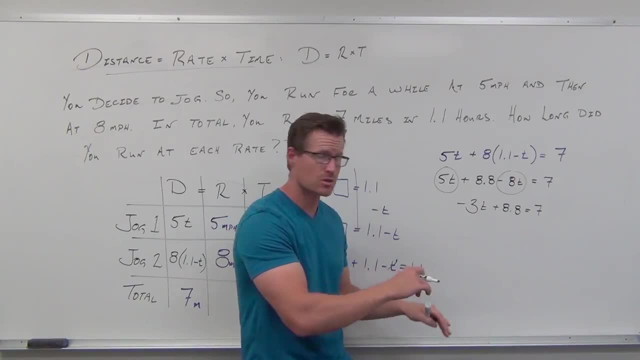 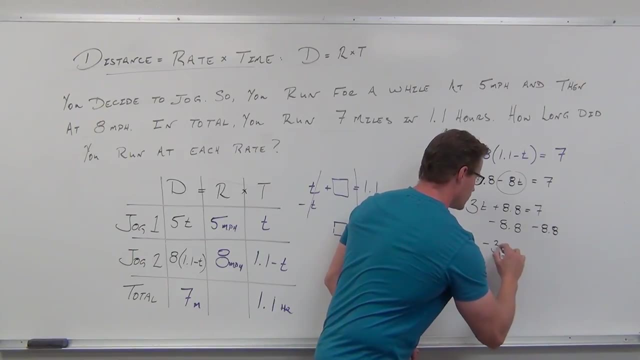 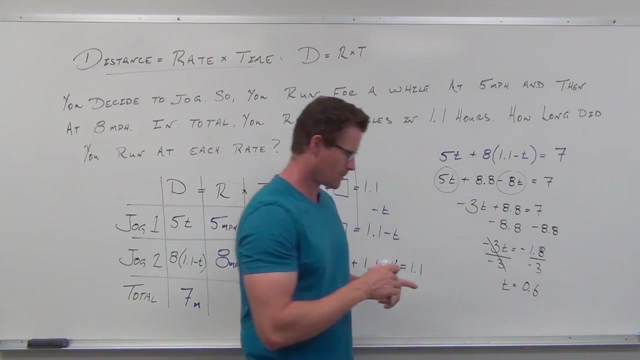 Our steps for linear equations say: get rid of the constant that's attached to your variable first, And your last step in linear equations is always divide. I'm begging you, I'm begging you, Please don't leave it here. Don't do that. 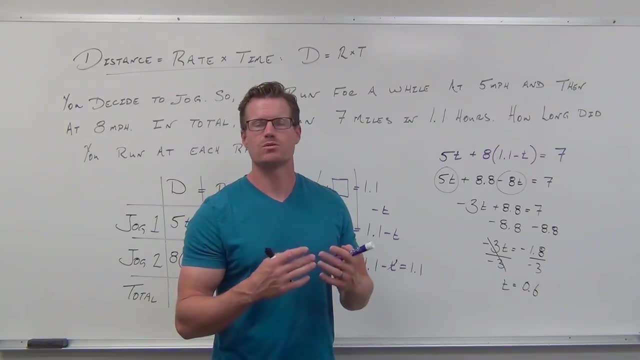 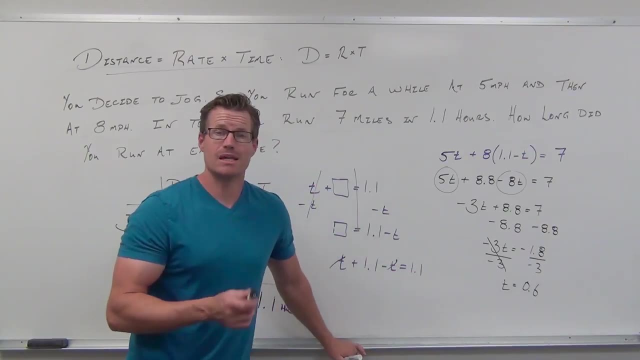 Don't do that to me, Don't do that to your teacher. Explain the problem. The whole reason why we do word problems is to answer real life stuff, So stuff that actually happens. So answer it. This question was: how long did you run at each rate? 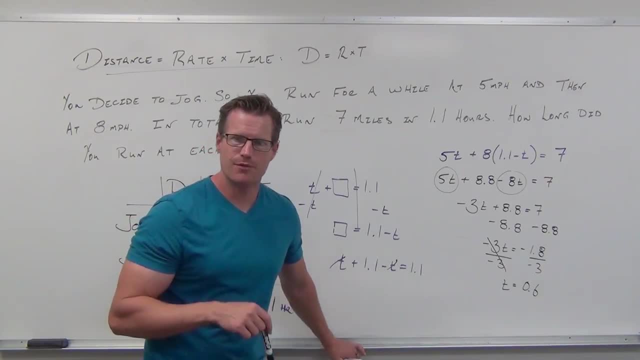 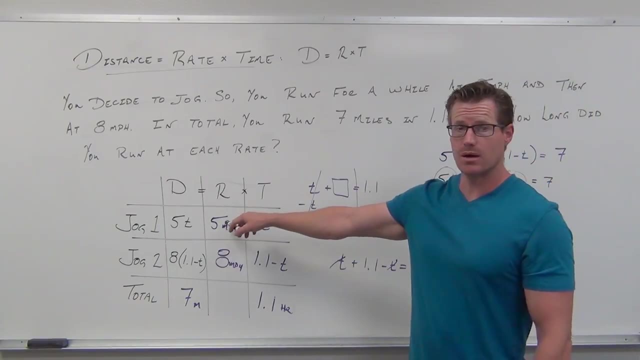 Well, look back at your table. It's all over the place. Why we did the graphic organizer? Look back at what the T represents. The T represents how long we ran at five miles an hour our first jog. Now what if you had reversed that? 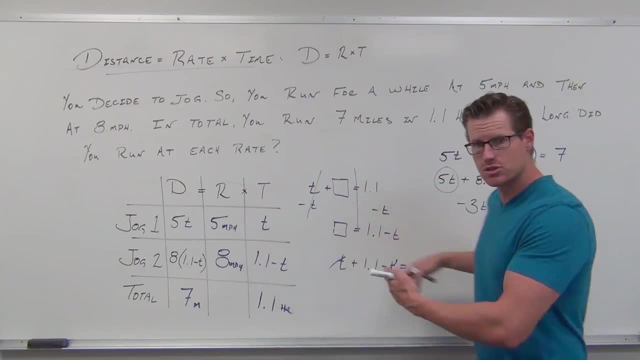 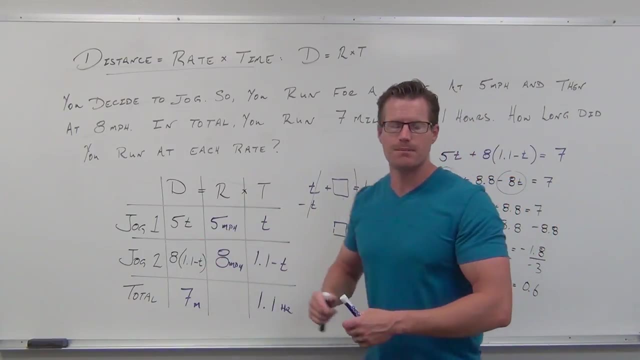 Put your T here, your 1.1 miles T here, That's okay. The T which you would have got would be different and it would represent the time for your second jog. It doesn't matter where you put it. It matters that you follow the process that I'm giving you. 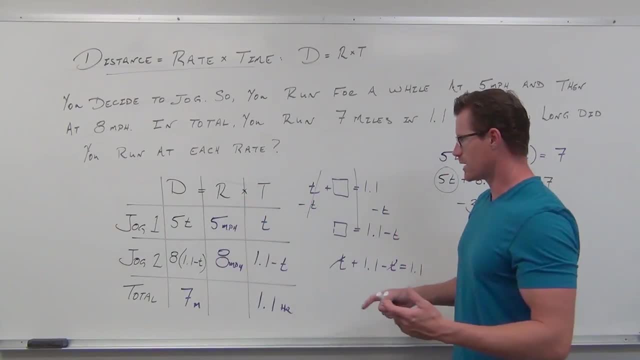 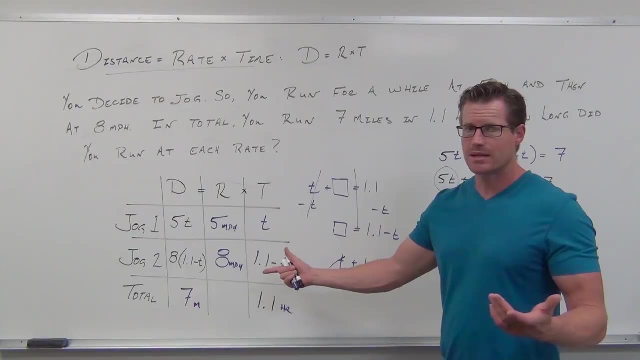 So our first jog was .6 hours. All right, So we have the first jog at .6.. How would you find out? the second jog, .6.. So it's given to you. Take 1.1 minus .6.. 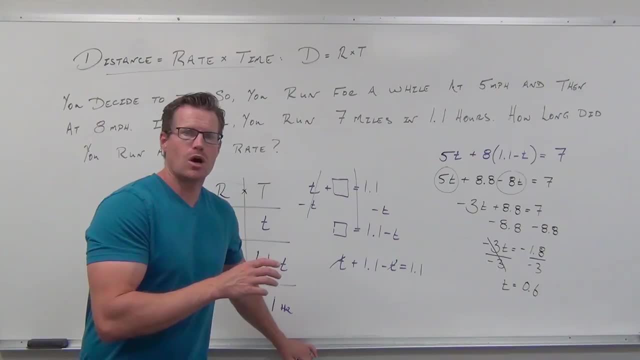 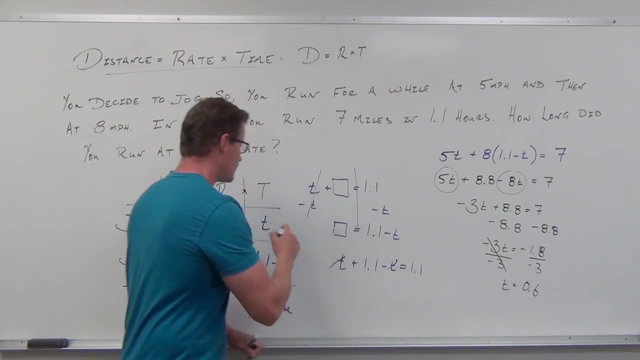 So our first jog. the way we write this out, you write a full sentence saying we jog five miles an hour for .6 hours and eight miles an hour for .5 hours. How would we get to .5? 1.1 minus .6 is .5.. 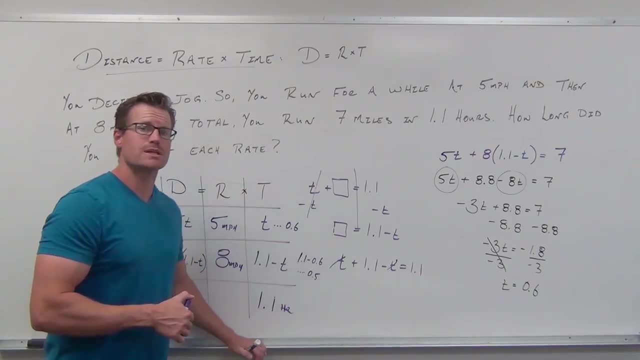 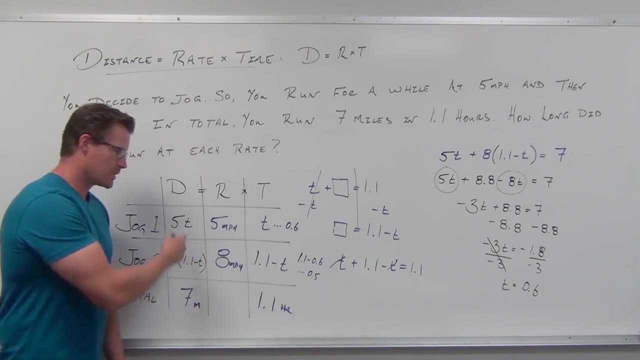 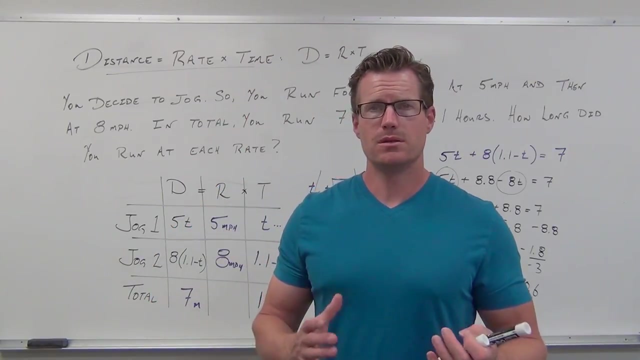 So we jogged five miles an hour for .6 hours and eight miles an hour for .5 hours. Look how it adds up: .6 plus .5 equals 1.1.. We used our distances to figure that out. Now. I told you a little while ago that I was going to talk about when you can use this differently. 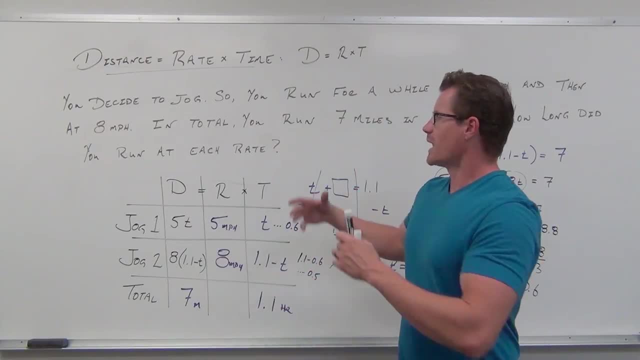 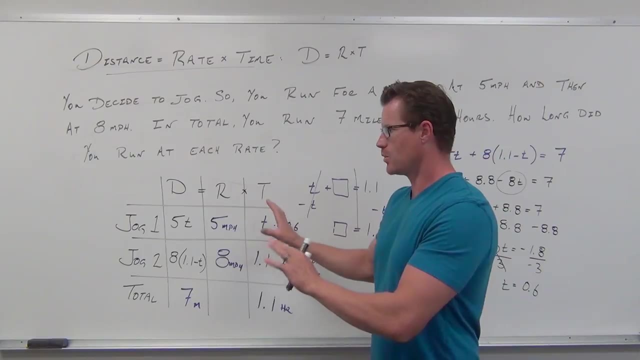 So let's say that we're not asked for a time, We're asked for a distance or we're asked for a rate. So check this out. You'd still fill out your table, What However you want. However, whatever information you're given to you, you're still filling that out. 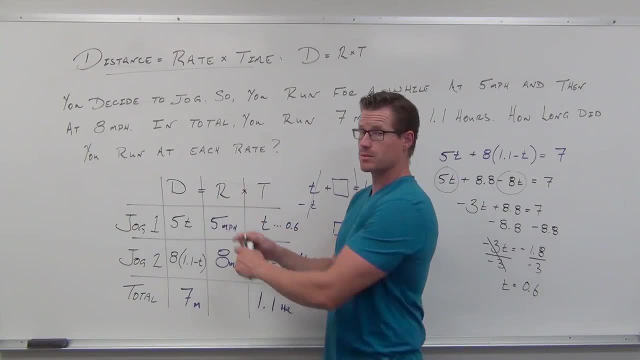 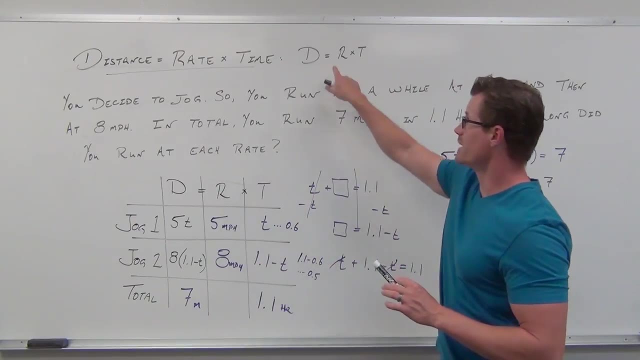 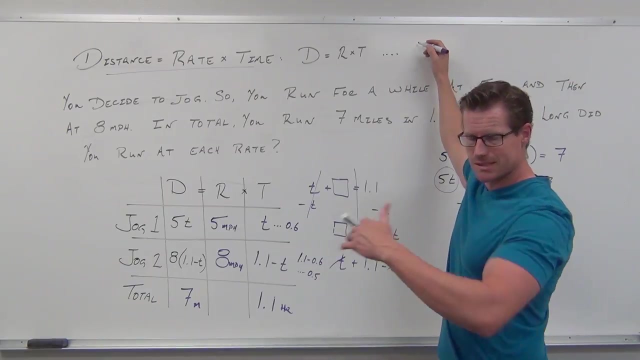 But we don't always have to go rate times. time equals distance. There's two other kind of permutations of this that we can deal with. If you solve this for r or t, we get two more formulas we can work with. If you solve for r, basically divide both sides by t. 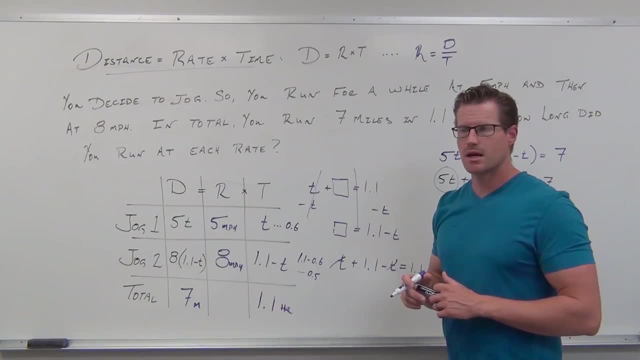 we can get that. a rate equals a distance, So divided by a time, Maybe that makes sense. If you went 100 miles an hour, I'm sorry. if you went for 180 miles and it took you three hours, you can figure out. you went 60 miles an hour. 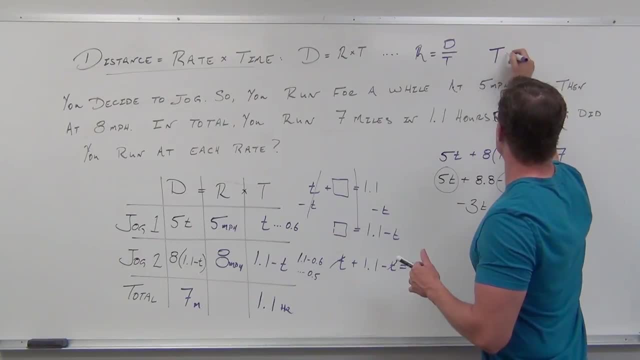 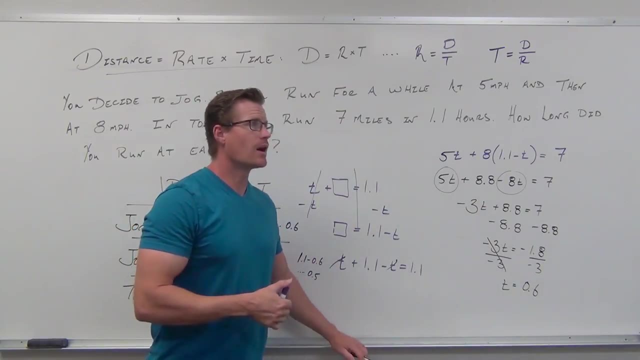 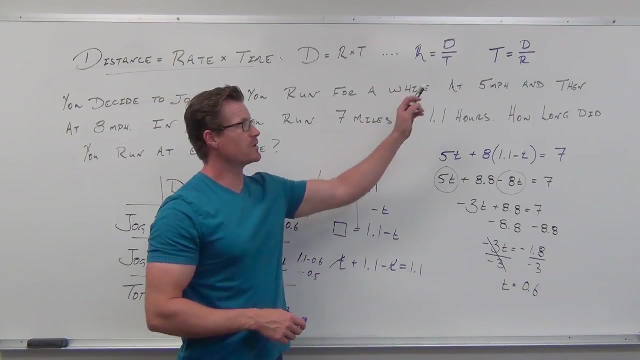 That's what that's talking about. If you solve for time, if you went 180 miles and you were going 60 miles per hour, you could figure out that it would take you three hours to do that. These are ways that we can. 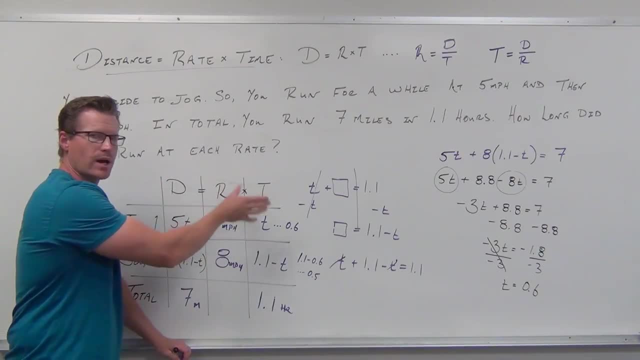 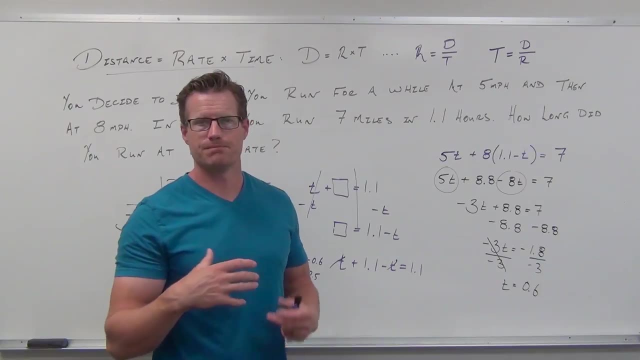 Use this table to our advantage. You can switch this stuff around, It doesn't matter. Maybe put time equals distance divided by rate. That's all right, But these are different ways that we can utilize this table. The big idea here, the hardest thing for students to grasp, is this idea.